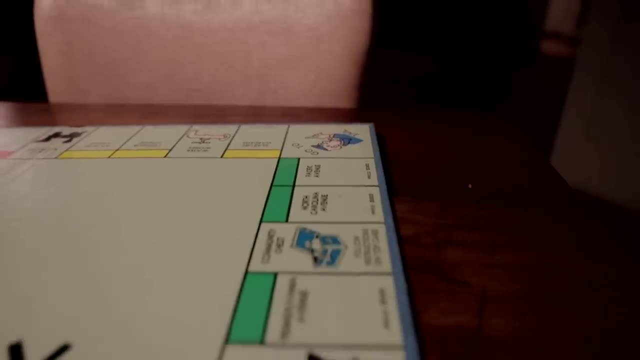 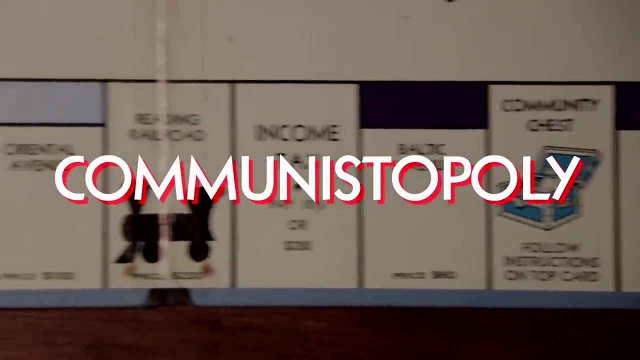 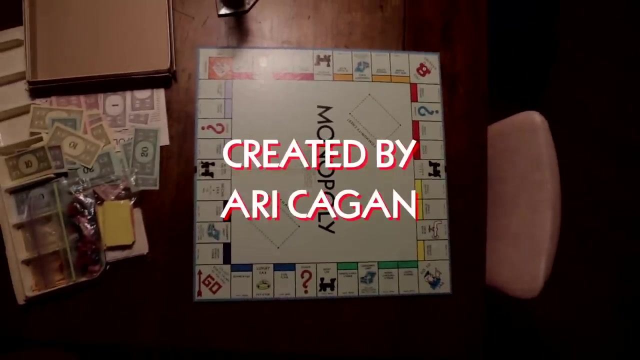 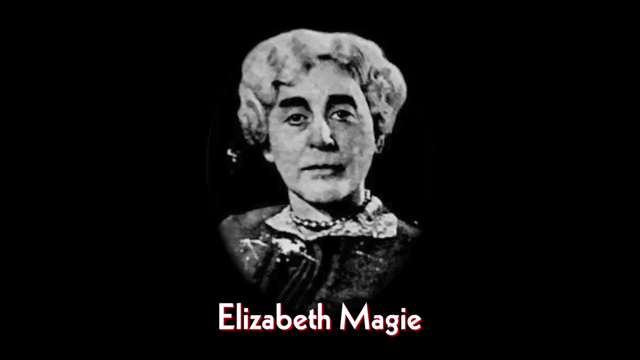 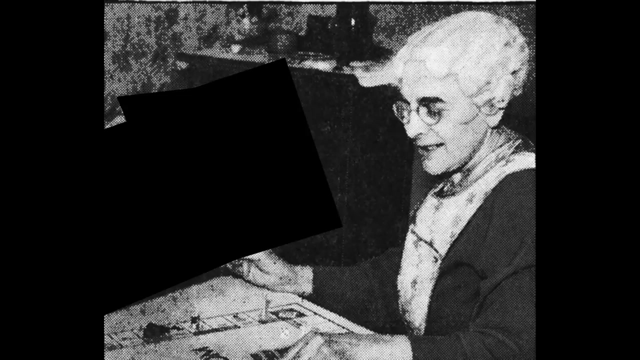 And then it dawned on me. Elizabeth McGee grew up in the Gilded Age and, after seeing robber barons get richer and the rest of America struggle to get by, she decided to invent a board game to educate people on how big business and monopolies are bad. 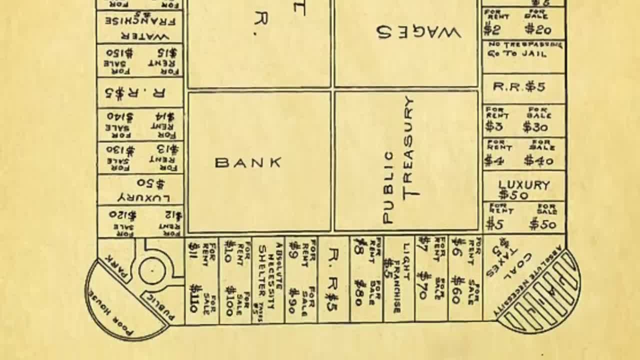 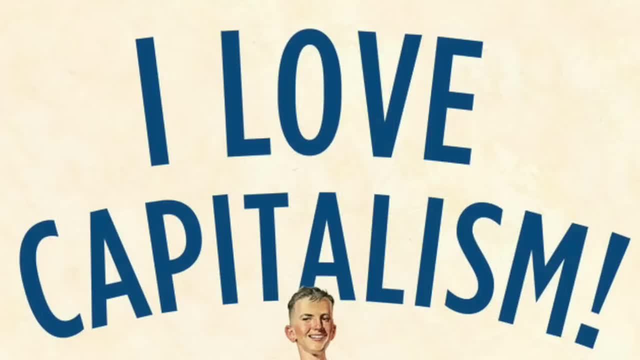 She called it the Landlord's Game and it was tremendously popular all across America. There were different game modes. You could play as anti-monopoly or monopolist. The second, of course, was the game everyone played. It was not uncommon for people to make their own boards. 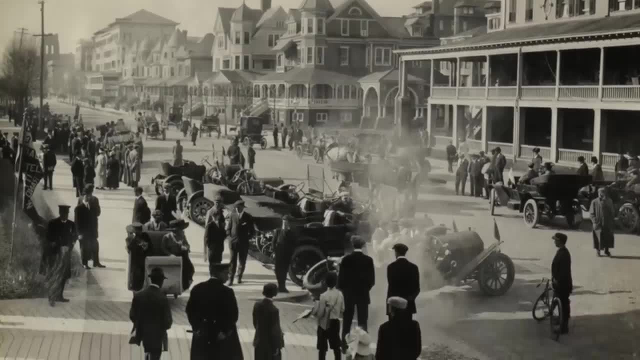 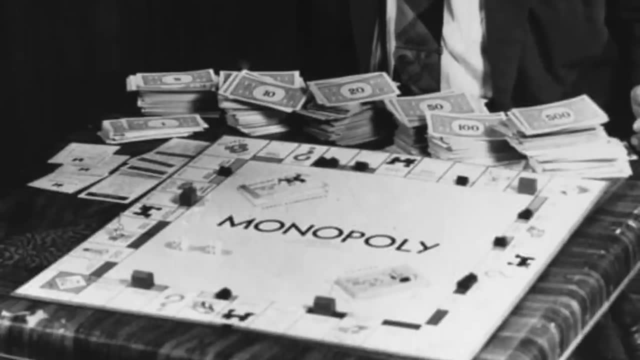 and in the early 1930s the Quakers of Atlantic City changed the names to match their local destinations. A few years later, Charles Darrow was at a dinner party with a few friends, found out about the game and made his own board. 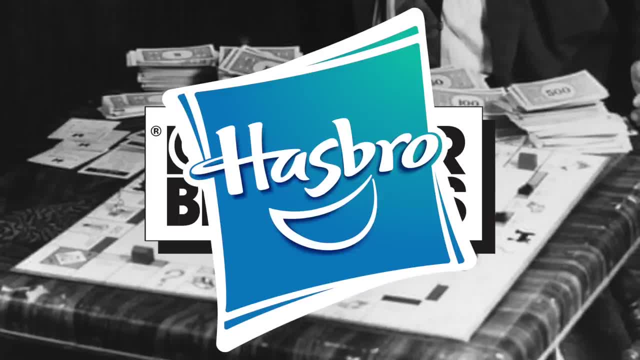 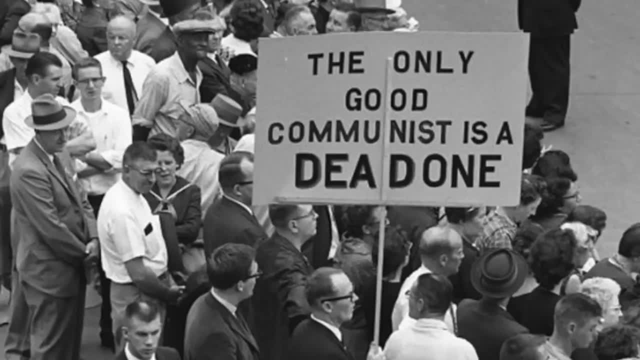 eventually selling it to Parker Brothers, who would go on to be bought by Hasbro in 1991.. Anyway, arguably Monopoly's greatest success came from being a capitalist game during the Cold War. It was a time of great prosperity for Americans. 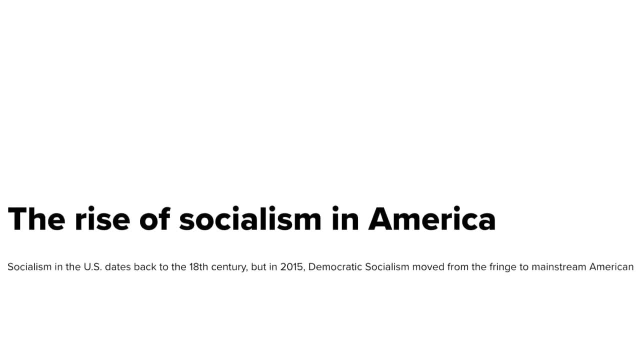 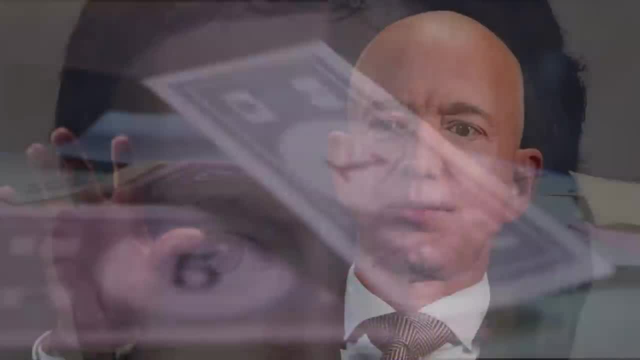 and the game greatly echoed that. But now people's views are changing. Perhaps playing Monopoly hits a little too close to home with the current businesses and politics of America. A game that during the Great Depression was considered a break from reality is now a hyperactive extension of it. 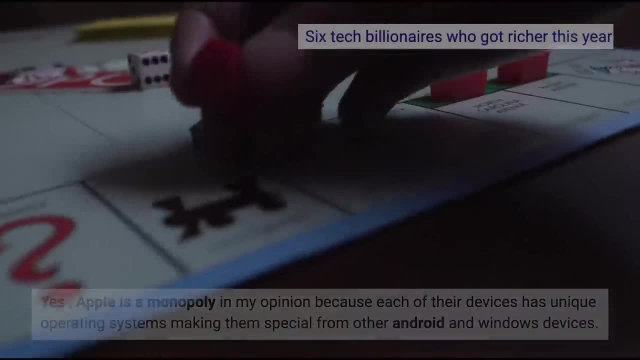 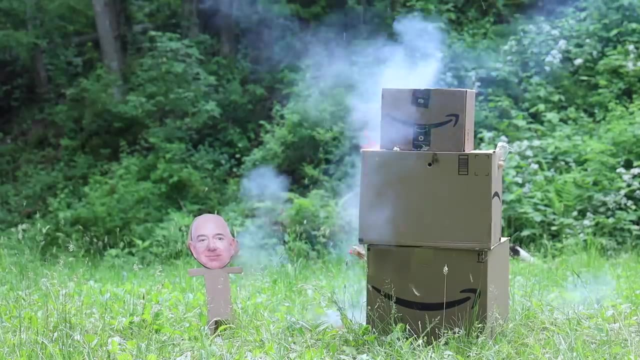 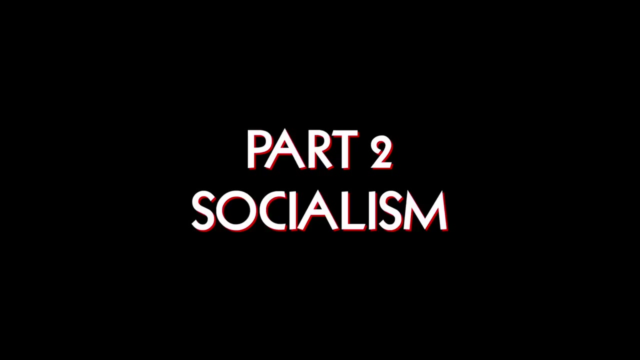 This new wave of capitalist rejection might cause people to hate the game that was once on their side. So, in honor of destroying the system, it's time to make Socialist Monopoly. So, as it turns out, Socialist Monopoly is already a thing. 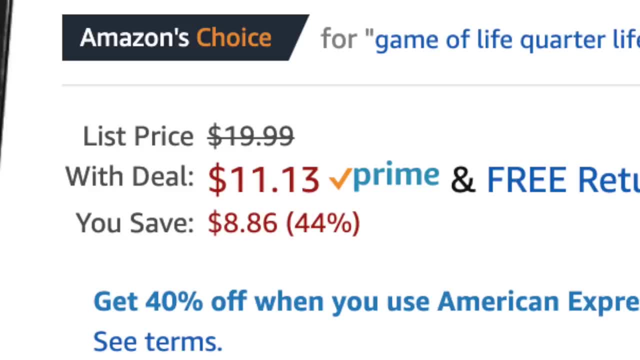 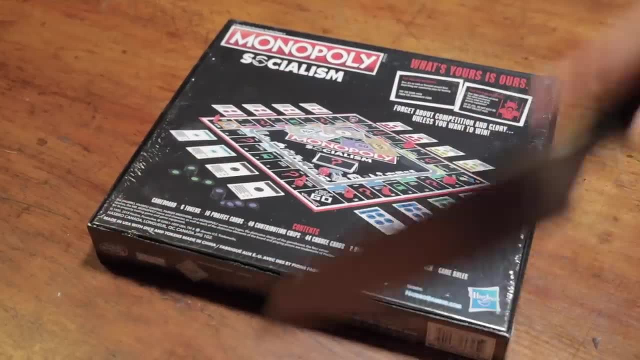 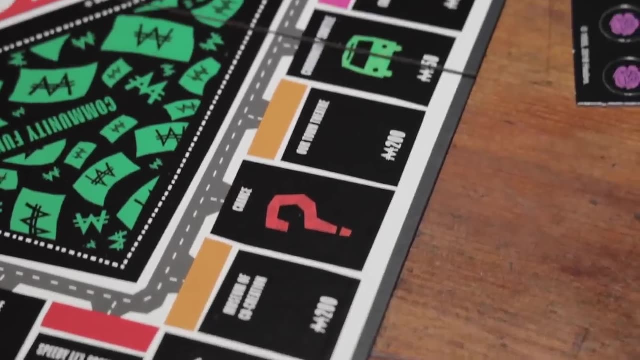 So I bought one On Amazon. It runs with the tagline: Winning is for Capitalists. I'm just going to cut to the chase here. This game exists purely to make fun of socialism, which I think is a bit of a chuckle considering our knowledge of the history of Monopoly. 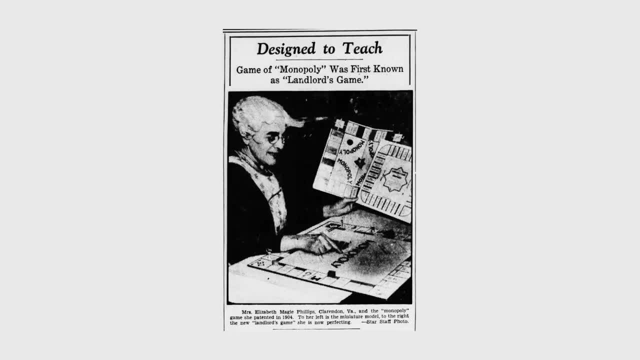 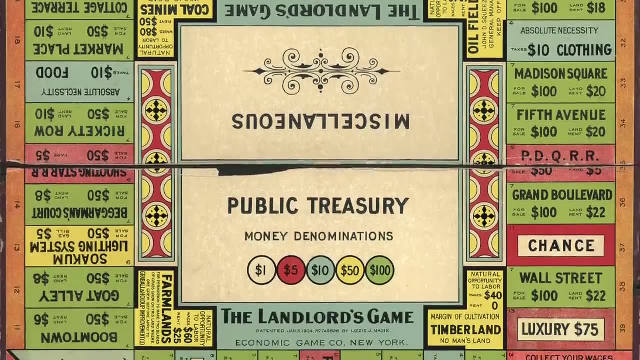 It really comes full circle. In 1903, when Lizzie McGee, an individual, first invented the game, it was about teaching people the perils of Monopoly and capitalism, And now we have Hasbro, which is kind of a monopoly. 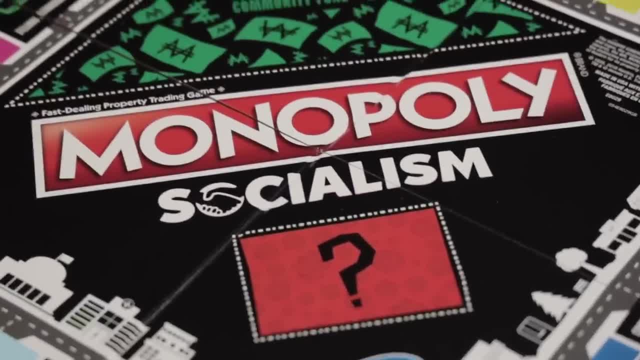 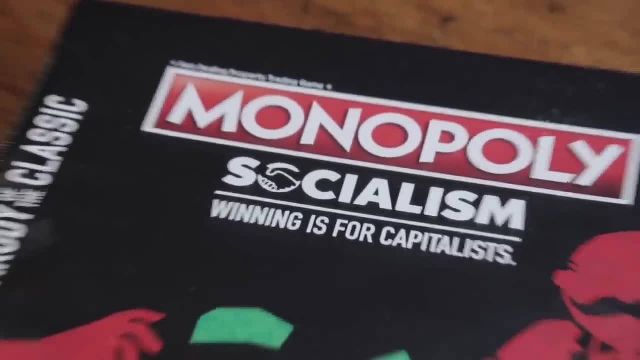 making a game about why socialism is bad. And it's not that I'm against making fun of socialism. I just think that it's kind of ironic, to say the least. There's also a really big part of me that thinks: why stop at socialism? 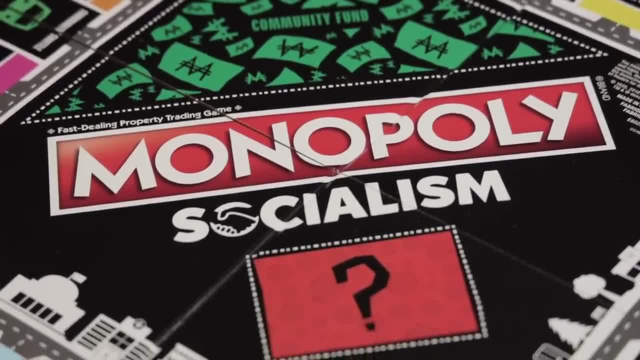 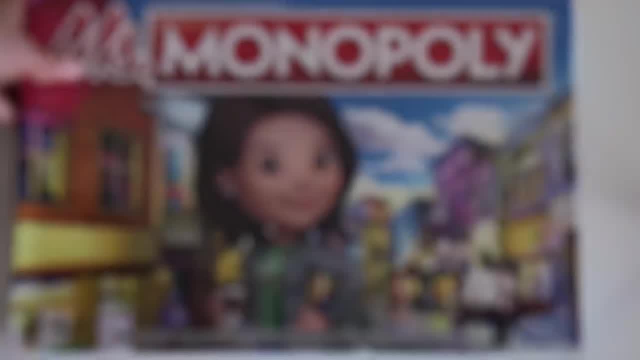 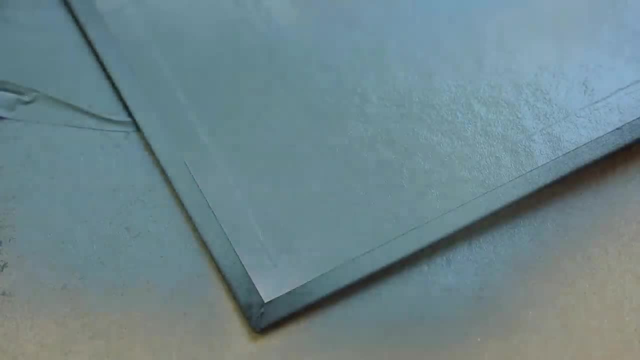 Like. I just feel that the idea could have gone a lot farther. I don't see too many real players saying that. I don't see that there's too much need to say. I think that the firstстра is the best solution. 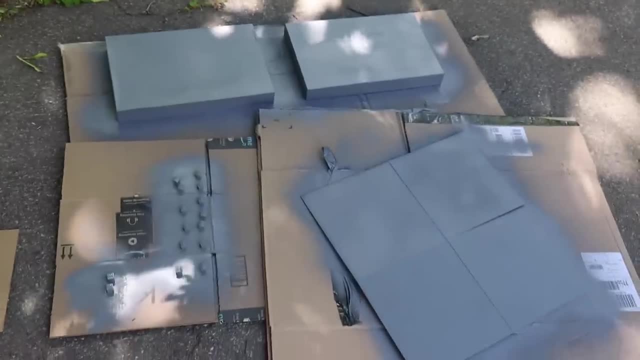 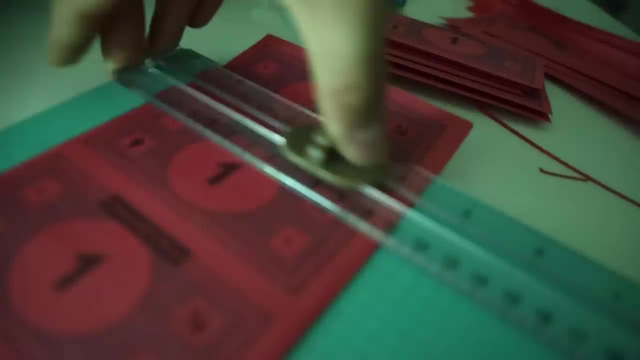 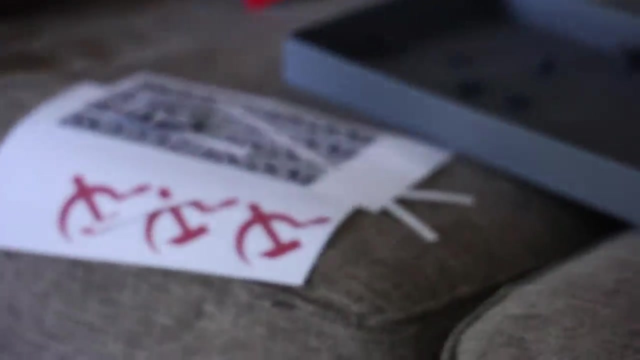 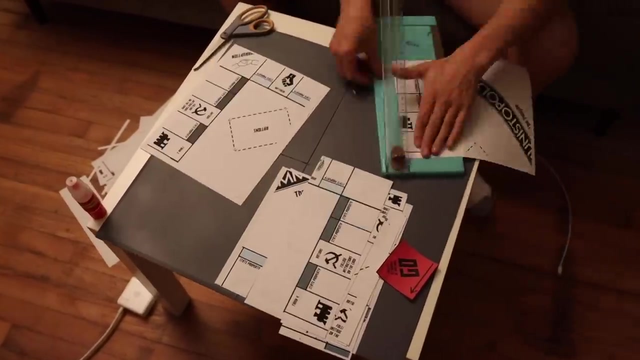 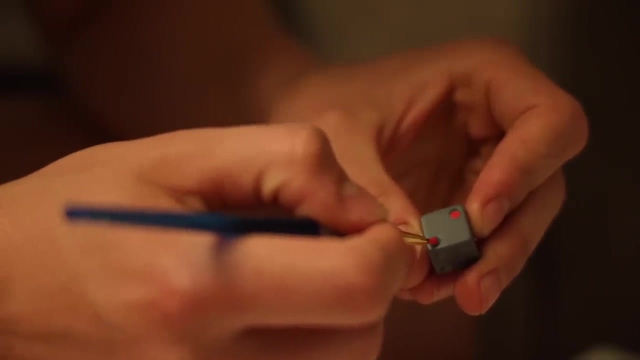 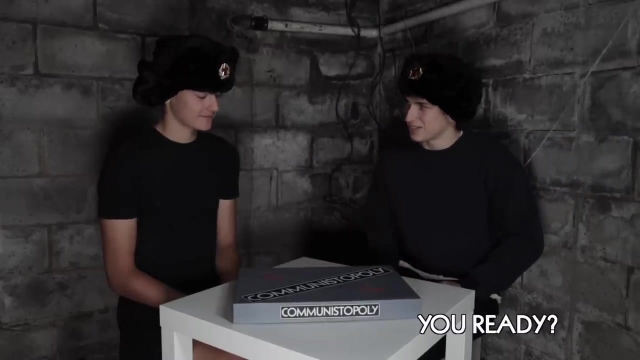 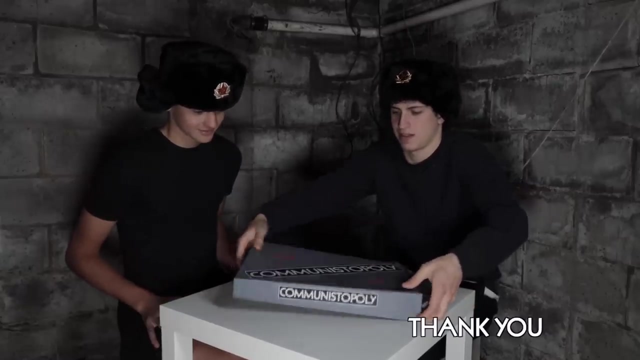 et daha, который va стать pire. Cuccccorcccccccccccah. There it is You ready, I'm ready. Okay, so of course, there's the box which is gray. It's very nice, gray, Thank you. 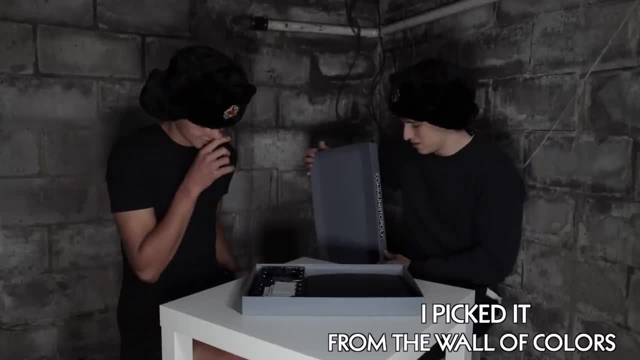 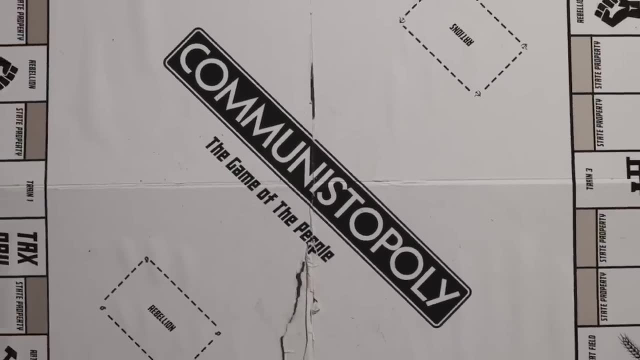 I picked it from the wall of colors, While that statement is factually true. I'm such an idiot I should have just said it was one of the 50 shades. Anyway, Communist Monopoly is very similar to normal Monopoly, except for a few key changes. 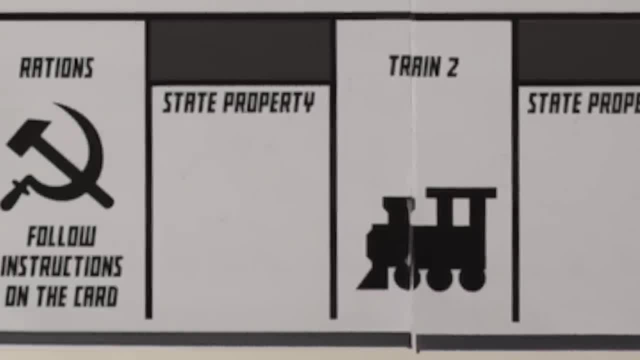 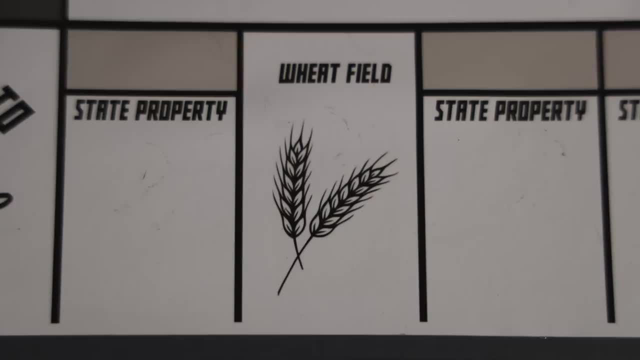 The first thing you'll probably notice is that the board only features state property, which makes sense because communism, Electric Company and Waterworks are replaced by Nuclear Power Plant and Wheatfield. Chance and Community Chests are replaced by Rebellion and Rations. 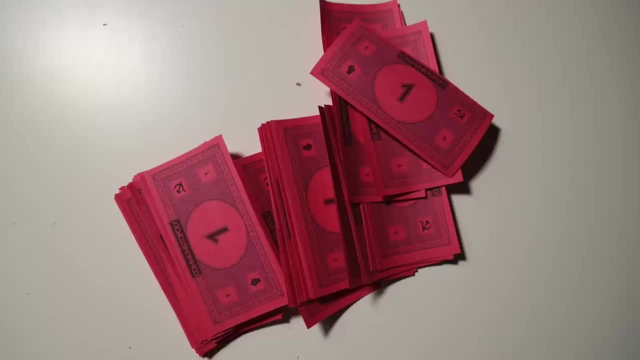 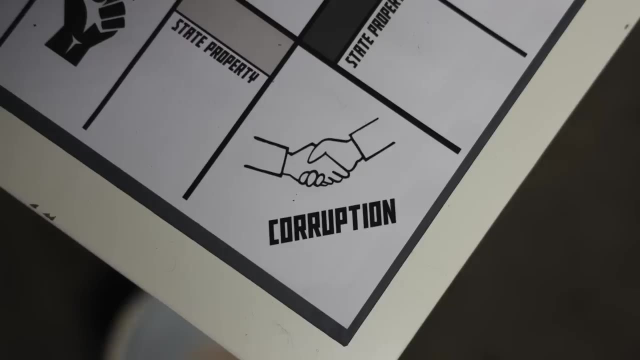 Every time you pass go, you only receive $2. In fact, this game only uses $1 bills because in communism there is no inflation. Free Parking has been replaced by Corruption. Should you land on this spot, you get to check another player's Rebellion cards. 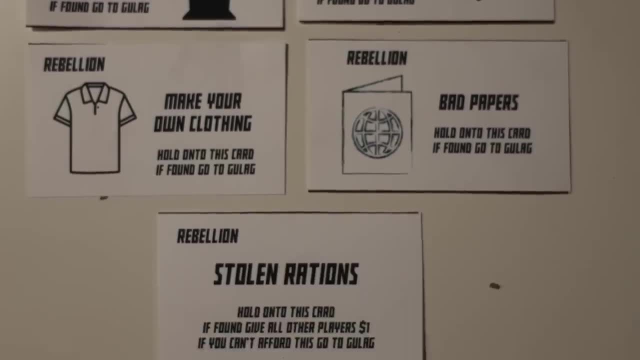 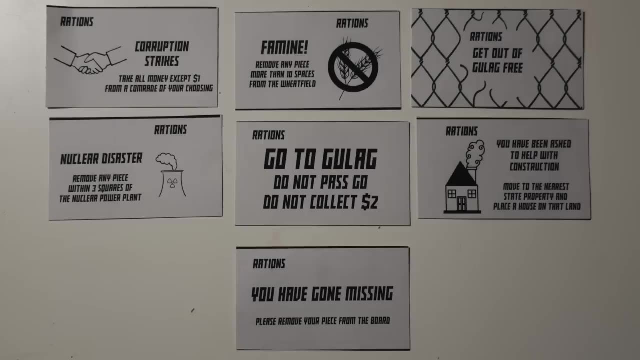 They will either be an enemy of the state and therefore sent to the Gulag, or they will display a Nothing-to-See-Here card which gets them all free. In order for this to work, you have to keep all your Rations and Rebellion cards, unless they explicitly state that you must play them immediately. 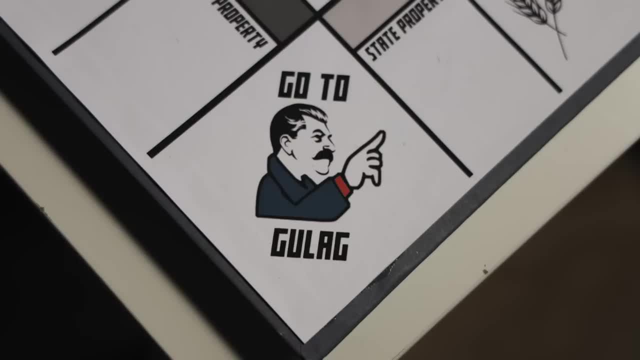 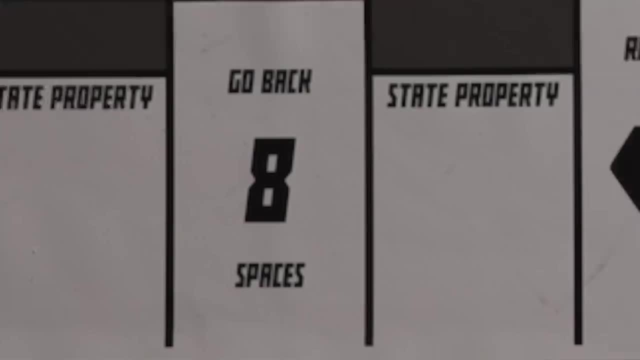 And last but not least, the Jail is replaced by the Gulag, With a matching style interpretation: Go-to-Jail spot. But wait, there's more. My absolute favorite spot, Go-Back-Eight Spaces takes you- you guessed it- straight back to the Gulag. 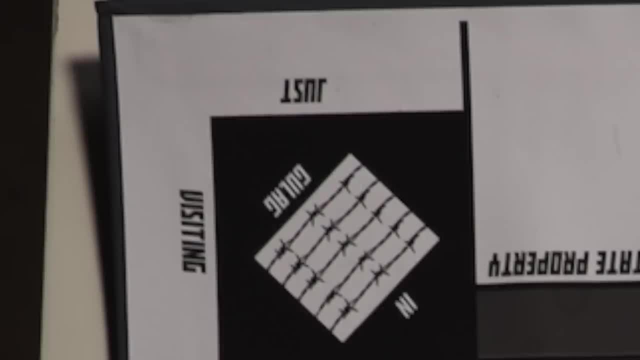 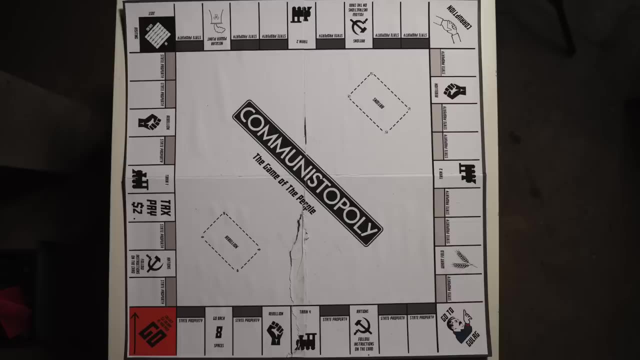 The Gulag is very similar to normal Monopoly Jail, except there is no three-turn rule implying that you could literally be there forever. The game ends when there is only one player left on the board, due to everyone else finding the meaning of life or mysteriously disappearing. 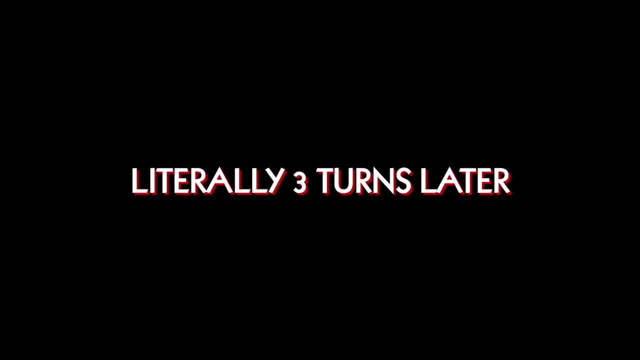 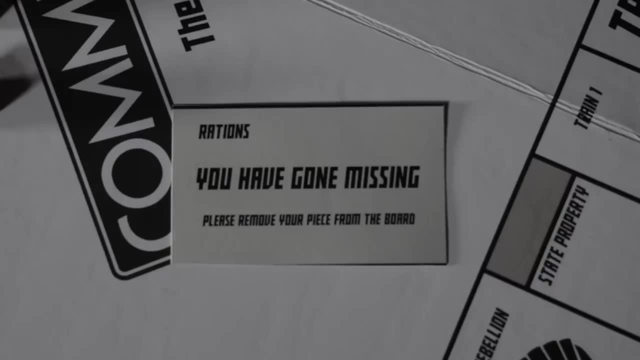 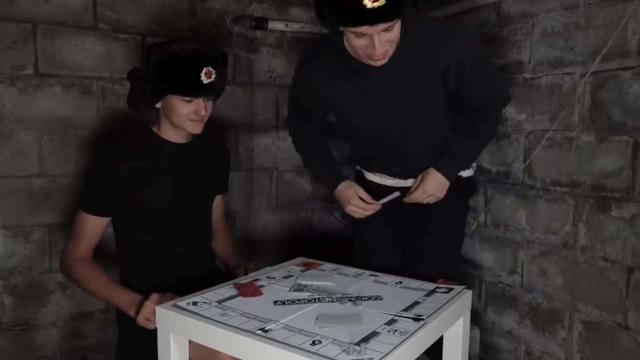 Five. Oh, I met you on the Corruption Square. Why is everything bad? You don't have a single good thing in the game. There's not a single good thing. I'm done, The game's over. And just like that, the game was over, so we decided to play again. 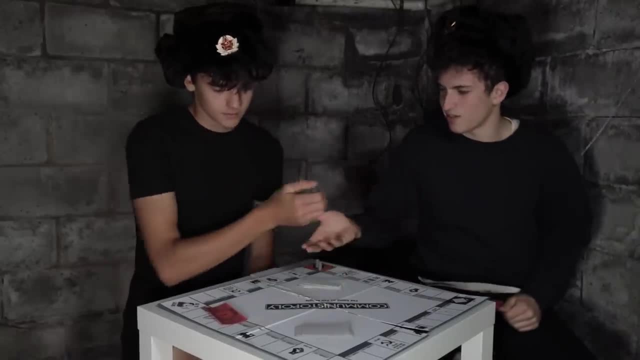 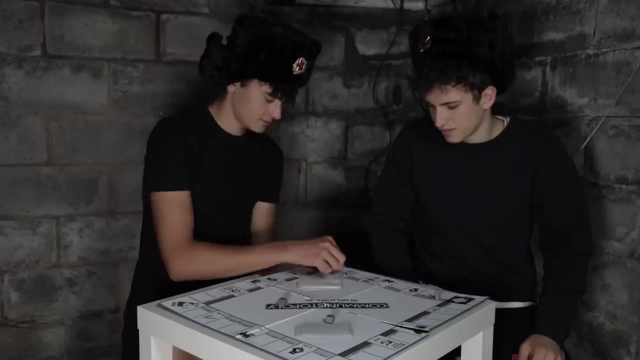 This time the game's creator will go first, because you obviously ruined everything Here, Because I obviously what Ruined everything, You were the one who died. Okay, let's not- Upon second playing, we realized just how boring. 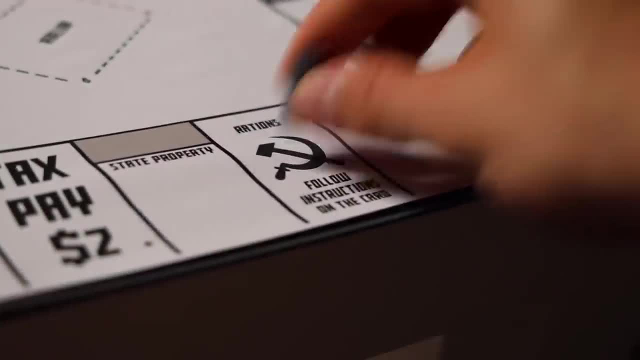 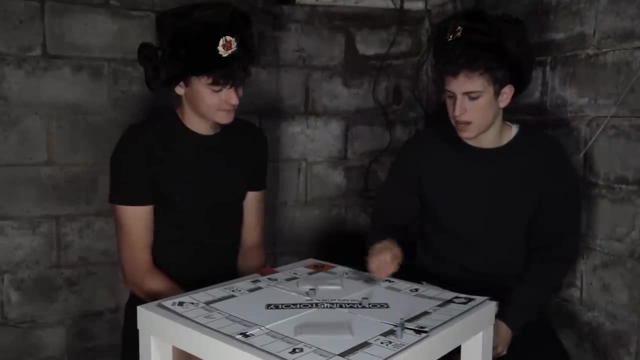 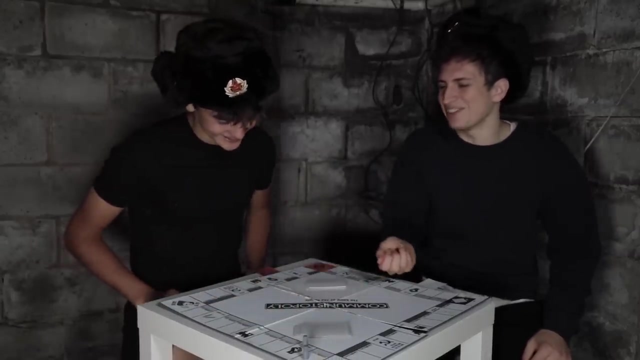 this game is Like There's genuinely nothing that happens. You just go around the board waiting for someone to mysteriously disappear, going from state property to state property, Which is exactly how I intended this game to be. A lot of what communism is about is removing greed and material objects from normal life. 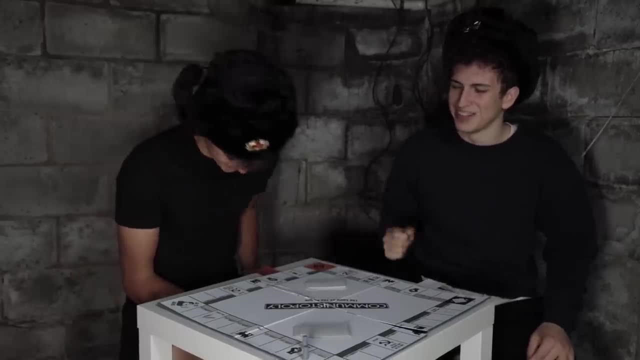 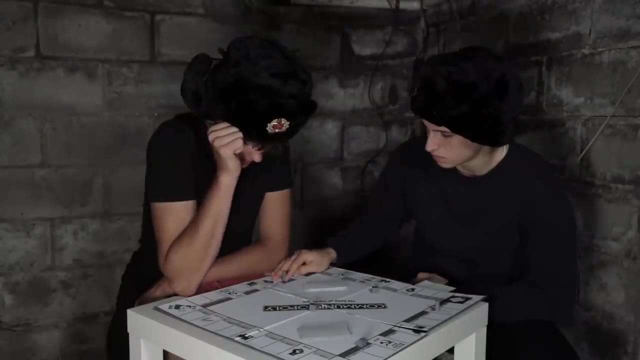 Forcing you to focus on what's truly important, Which, if I'm being honest, I feel like I've perfectly executed here. I've made something so boring that it forced Max and I to focus on life's truly important things. 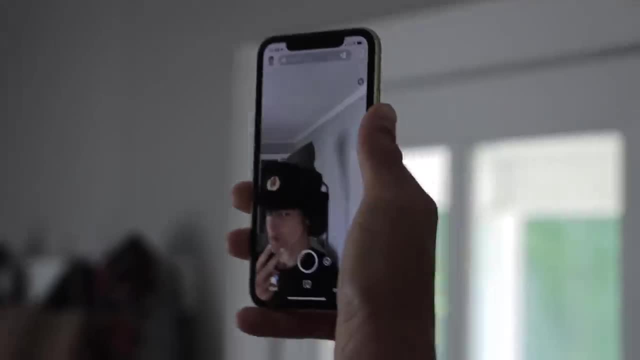 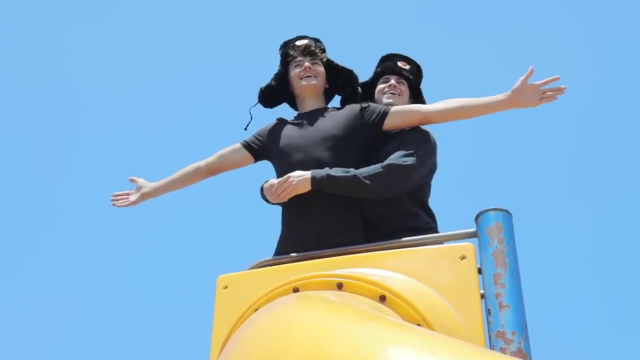 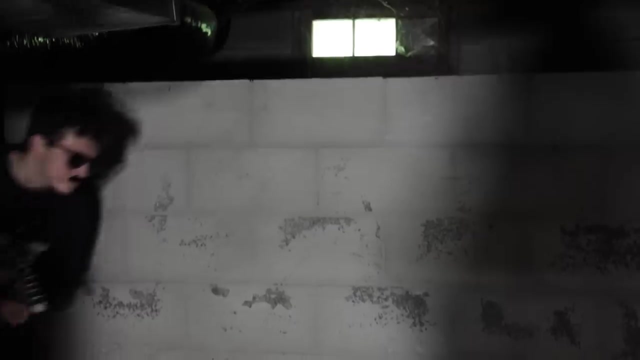 Like art, science and the meaning of love. So the next time you're about to call someone a commie bastard, maybe hear them out, Because communism is actually hella dope. You're both under arrest for treason and 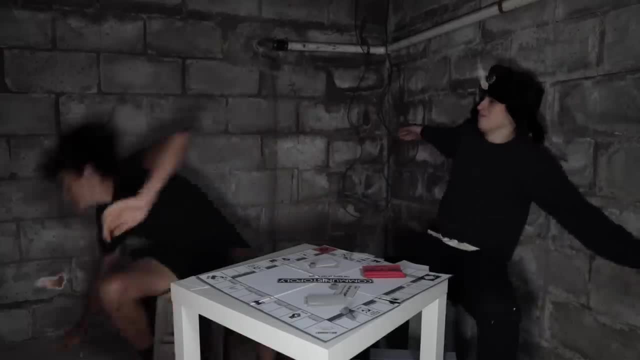 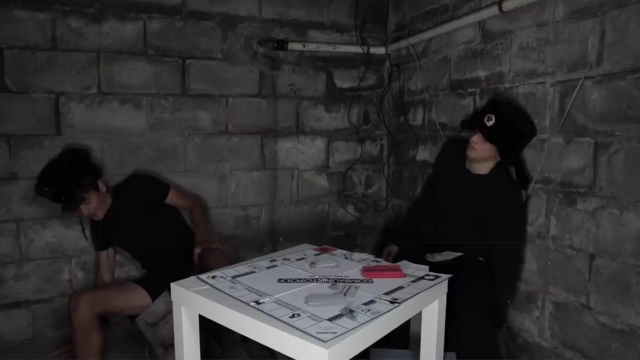 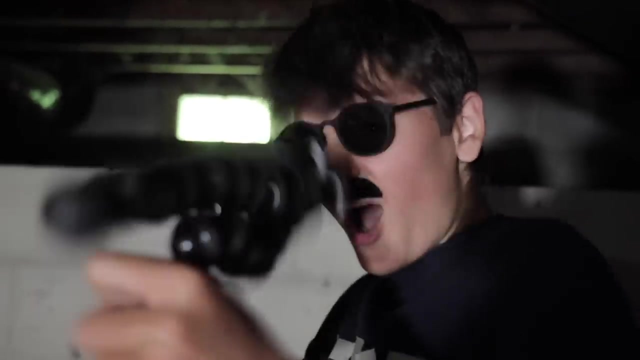 whatever else And where at least I know I'm free And I won't forget the men who died, who gave that right to me, And I'll have his head up next to you and defend her still today. 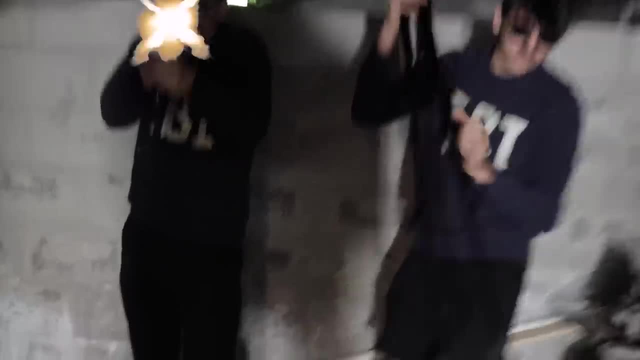 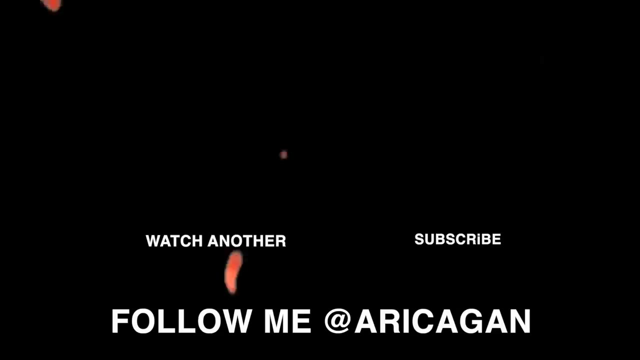 Cause there ain't no doubt I love this land, not just the USA. Subtitles by the Amaraorg community.